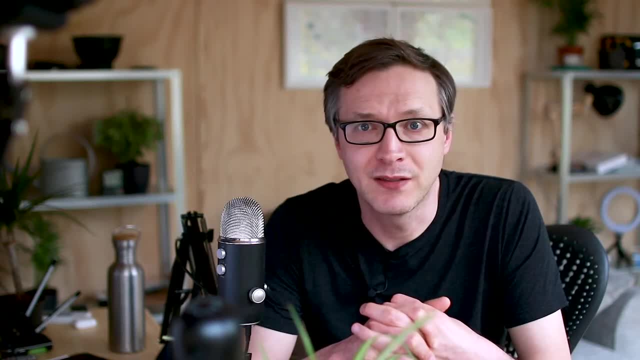 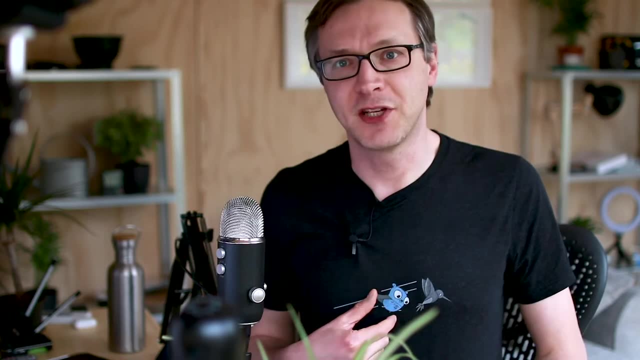 And therefore the caching plays a really, really important part of how things play out in the backend. But before I begin, check out my new t-shirt. I've got this kind of goofer character chasing the Superthread hummingbird. If you guys want to win one of these t-shirts head to 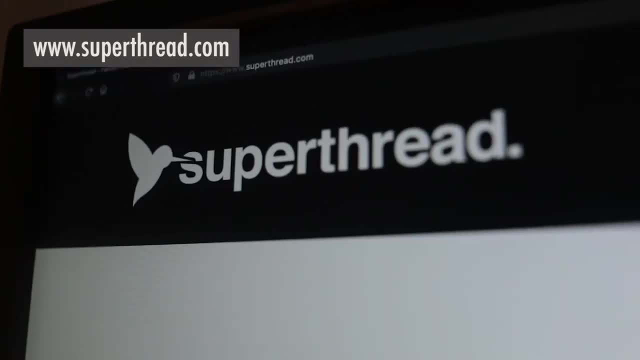 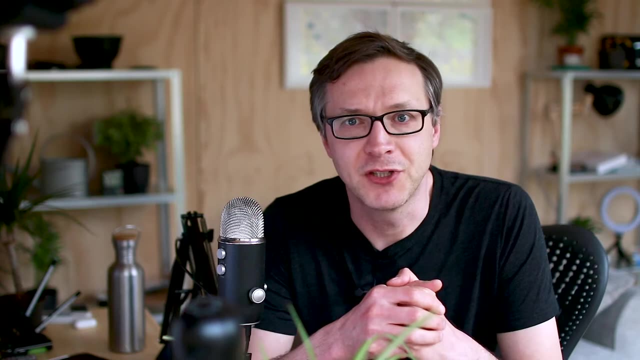 wwwsuperthreadcom and sign up for early access. We are looking for early access subscribers so you guys can test out our early product and give us some feedback. We'd really appreciate it. Anyway, without further ado, let's go through different types of. 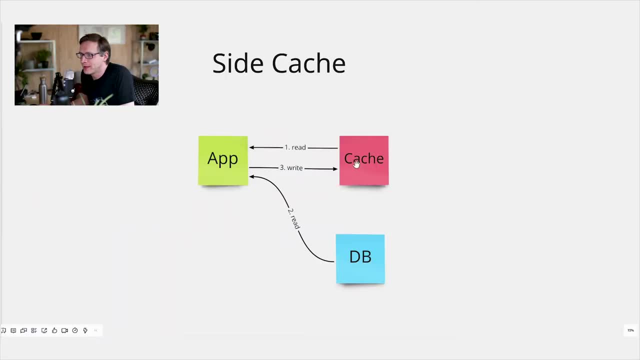 database caching. So, to begin with, the way caching is typically done is by using a side cache approach, And the way that normally works is that you would have your backend app written in something like Java or Golang or PHP And that thing would try and access data from the database. 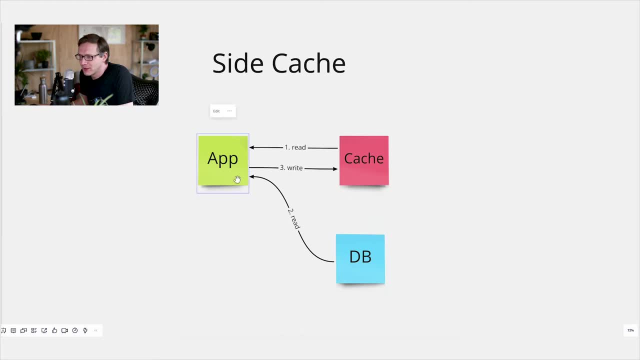 here. But the way the flow would normally work is that you'd kind of have a cache in front of the actual database, So the app would go and try and read the record from the cache And if the record doesn't exist, then it goes basically and reads the record from the database And then it hydrates. 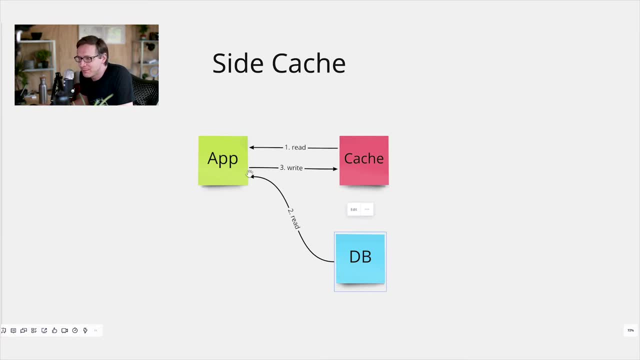 the cache itself, So everything is done basically by the app itself, So you have to program this logic yourself. This is a pretty solid approach And basically I think it's the most common approach and a lot of people use it And it's a really nice approach. The issue is when you have 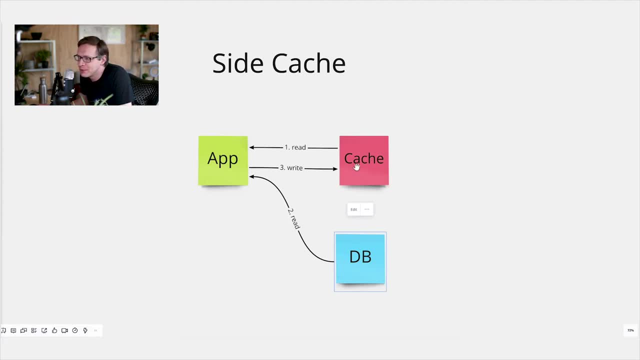 records inside of cache. how long do you keep them in there? How often do you have to kind of go to the database And rehydrate the cache? These are some of the things you have to think about, And it may be a little bit easier with kind of straight records where you kind of just get kind of a user object. 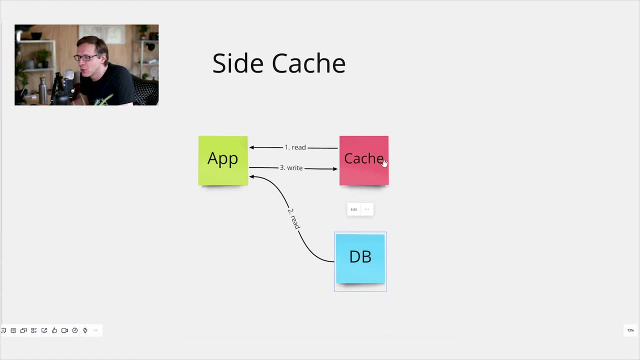 But when it comes to queries, you know like, let's say, you update a record which affects the query, you then cache the query in here and so on and so forth. So you can get really complicated really fast. But let's say, to implement a really simple version is not that difficult. 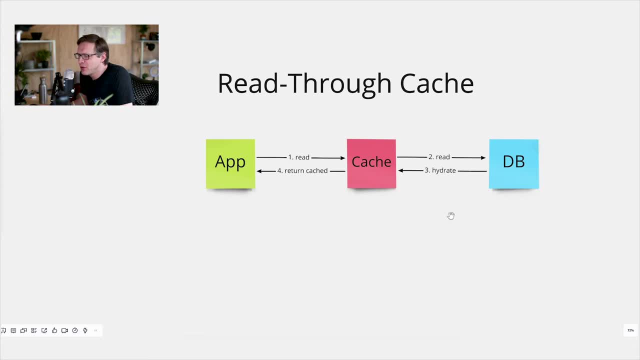 The next approach is read through cache. So read through cache is a feature of the database And it's a feature that's offered by some databases. So you kind of this is the way it kind of works. So this is your app, let's say a PHP or like Golang app, and then it kind of tries. 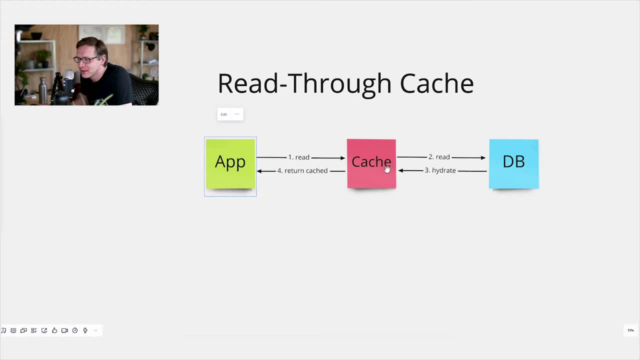 to read the record from cache And if the record doesn't exist, the cache itself. so if this is part of the DB. now, you see, so this is no longer being done by the app. So the caching kind of layer of your DB then goes and reads the record from the database and then hydrates the cache and then 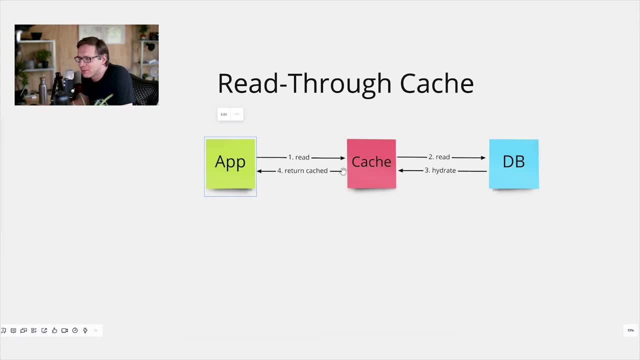 cache records. So then basically, next time somebody comes they'll have the cache record here inside of the cache automatically. The same thing goes for write through cache. Once again, you have your app and it tries to write the record and then the cache layer of the actual 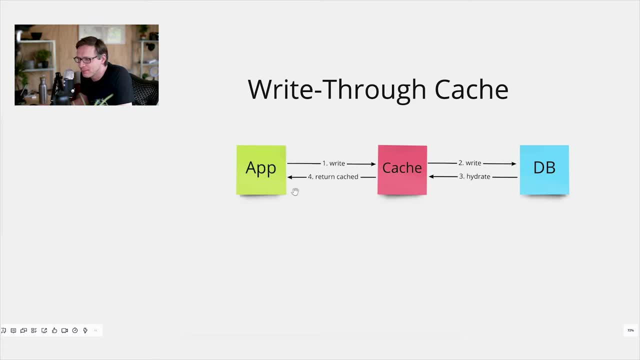 database. So this is part of your database application. This isn't done by your app. once again basically says: let's write this to the database, which is basically writes it on a hard drive somewhere, And then basically let's get this record. 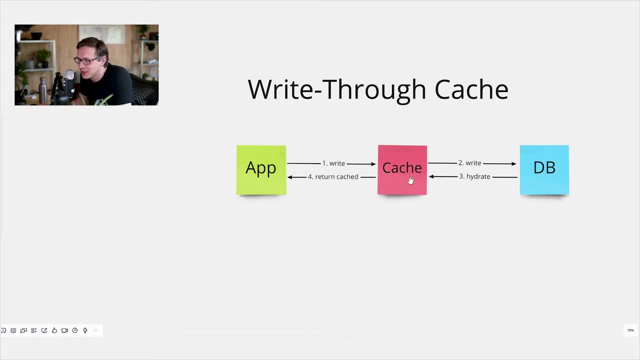 from the database and hydrate the actual cache part of the database. So once again, this is all done by the database, So you write the record. then the caching layer kind of says I don't have this record And it says, Okay, I'm going to write this record to the database And 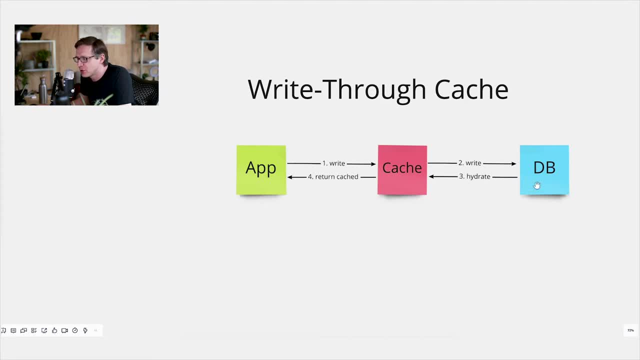 then I'm going to pull, pull the actual written record, the record I just wrote back into cache, and then the actual record is returned to the app from the cache. The next scenario is the write around cache. Okay, so this is the way it works, Rather than 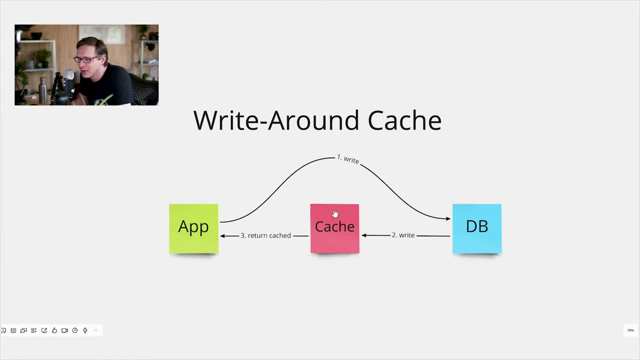 going through the caching layer. you kind of go around the caching layer. Okay, so the caching layer basically is not your app. it may be part of the database. for example, say you know, Postgres can have this caching layer. So what you then do is you the app, or your app goes and 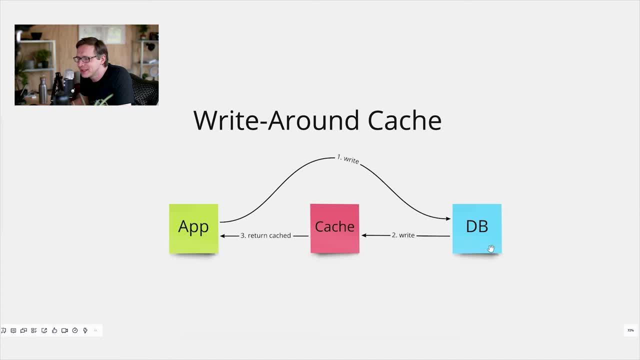 writes the record to the database straight away And then the database itself then populates this caching layer And then when you actually go and get the actual record, you get it from the caching layer of the database. You don't actually write through cache, you write around cache. Okay, And the last scenario is: 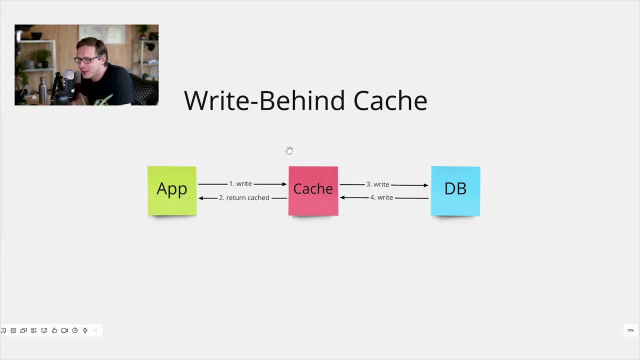 right behind cache. So this is really the dream. you know like so. but the problem is like if this kind of part here breaks, then you have problems, because or you may write something to the caching layer of the database And then the caching layer returns this cache record and says: Oh it's. 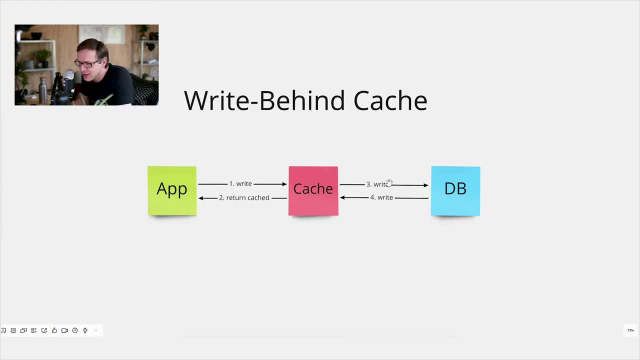 written, And then it goes behind the scenes and writes it, writes it to the database and then kind of writes it back To the cache, rehydrates it, back back to the cache. Now the problem here is that what happens if you write to the cache and then the cache flakes and then, and then the cache says, Oh, I've written the. 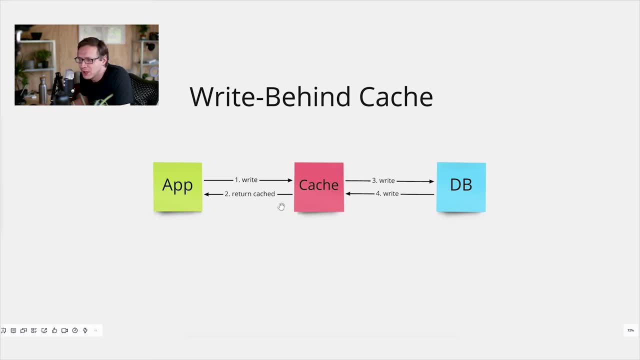 record And then just after it says I've written the record flakes out, then it doesn't get written to the database. So basically then you have kind of consistency issues. So in such cases basically what you have to do is have many kind of notes of the actual cache replicated, So in case one flakes. 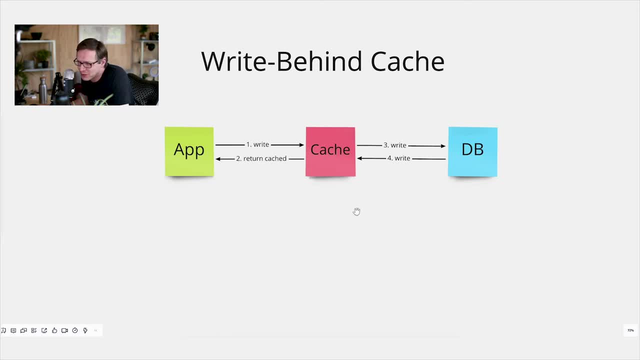 out. basically you have more reliability because the other one is going to do the same thing. So this is kind of the ultimate dream, And then also in such scenarios, you may have actually the caching part, So the in memory part. do your queries too, which would be really cool. So it kind of 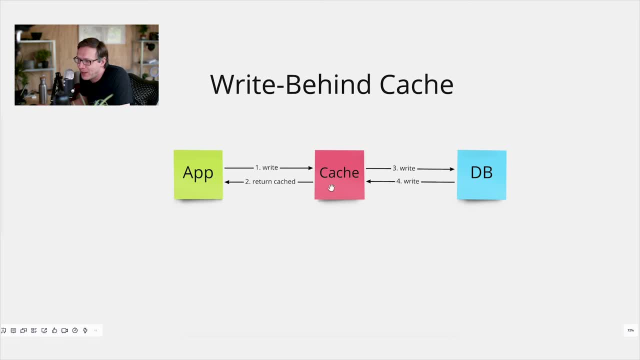 it's kind of a replica of what's on the hard drive And that's the ultimate. But then, once again, as I said, what happens? if there's this break between the actual memory and the actual hard drive, then you kind of have these inconsistencies and it can cause kind of a. 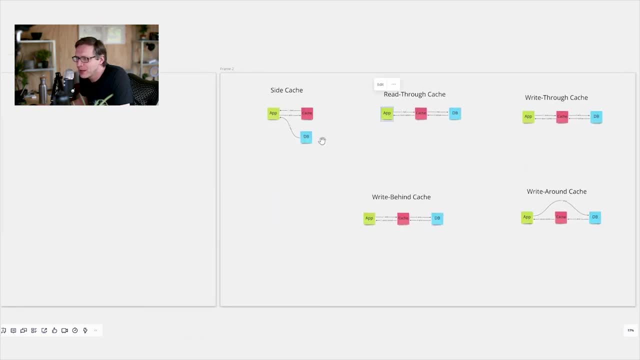 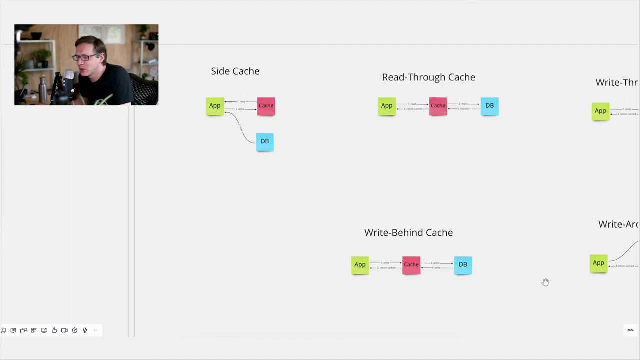 nightmare. So what do you kind of choose? It all depends on what you kind of are happy with. Do you want eventual consistency Or do you want immediate consistency? Is writing speed important to you? Is reading speed important to you? How important is reliability? Are you talking about the bank? 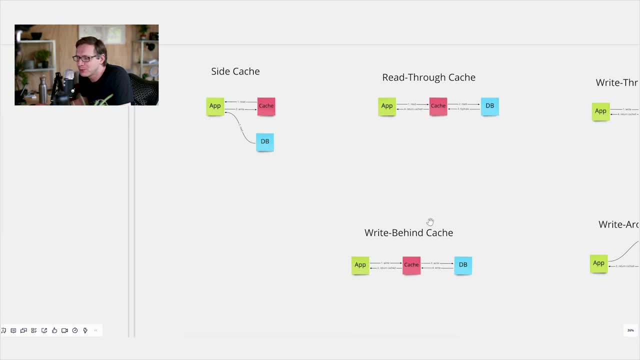 here. I mean, must the record go through? Must the record be absolutely consistent? Then you kind of have to make sure that the record gets written inside of the database. But then you see if the caching part of the database, for example, 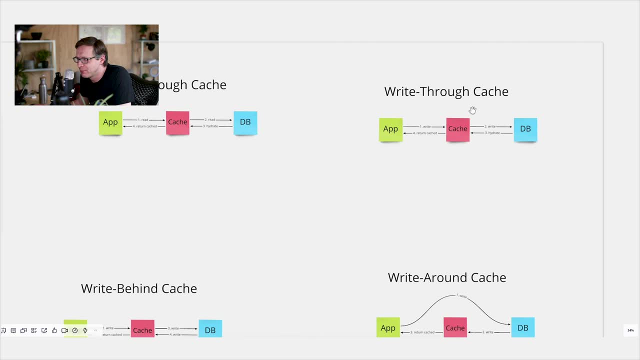 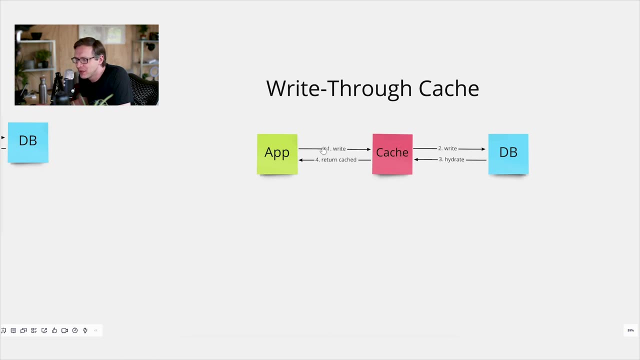 let's say you kind of you do a write through here. for example, let's say you're a bank and you do a write through, So you have this caching part basically on the database, which then receives the record and then writes it to the database. Normally what happens is that. 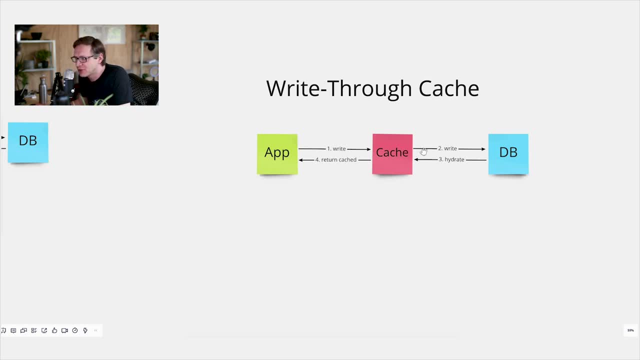 this caching part sits on a different machine, So you have this kind of extra network hop to actually deal with. And then, especially if you have replicas on the actual database side, on the hard drive side, and if you want absolute consistency, ie.